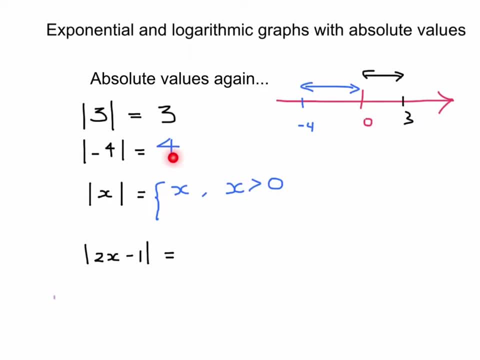 we multiply it by a negative 1 to get the positive version. So in other words we write: it's equal to negative x if x is less than 0, or if it's or if x is negative in other words. And we put in that little equals there. 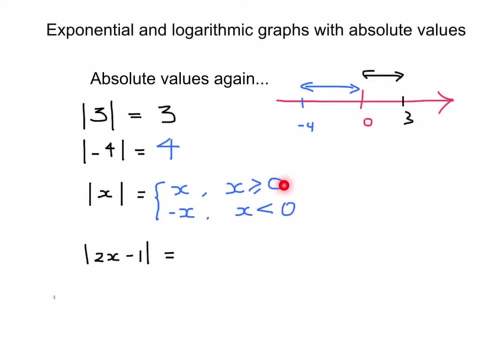 to make sure that we cover the equals case when x equals 0.. Now just one other one. If I have anything inside that straight bracket, we can split it up into two pairs of scenarios. Scenario number 1 is where the stuff inside the square. 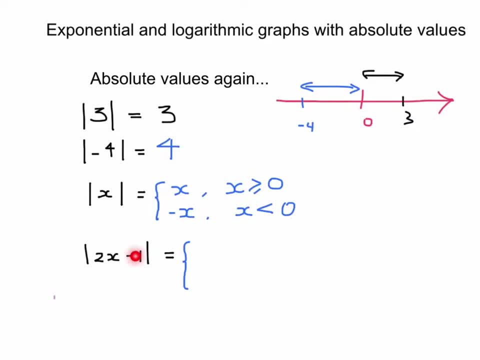 the straight bracket is actually positive to start with, That means you keep it the same if that thing was greater than or equal to 0. And the second scenario is: if that was negative in the first place, then you have to multiply all of this by a negative 1.. 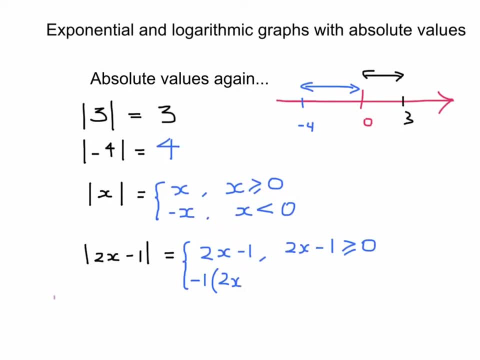 So we can say negative 1 times 2x minus 1, in the scenario that 2x take away 1 was negative. Now obviously there'll be requirements of rearranging this section of the limits so that x is actually some sort of. 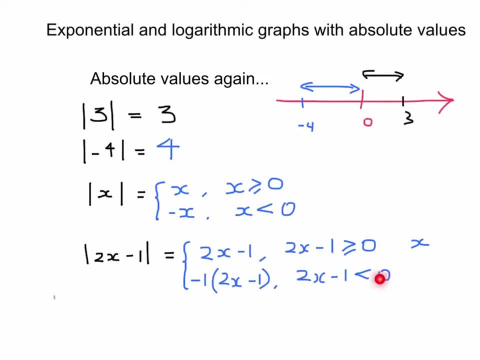 interval. But I'm going to leave that for now because that's actually less important. But for the purists, here's what you should get. You should get: x is greater than or equal to 1 over 2 in the first case. 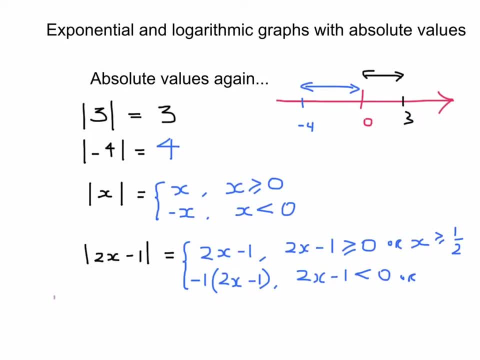 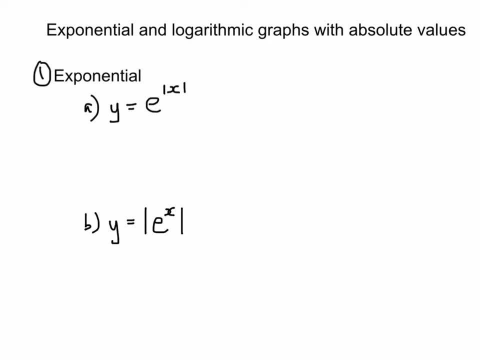 And in the second case, the opposite scenario: x is less than 1 half. So on to exponential graphs with absolute values. So what we look at is writing this initial equation as the two separate areas, So you will have the scenario where x was positive. 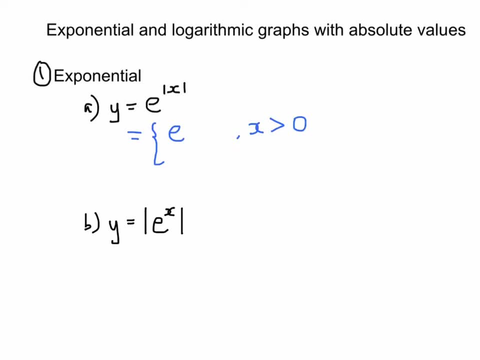 and that's when we keep the x as x, over here as the index. The second scenario is where x is negative, in which case we multiply this number by a negative 1.. So when we draw this graph, you'll actually have two parts to it. 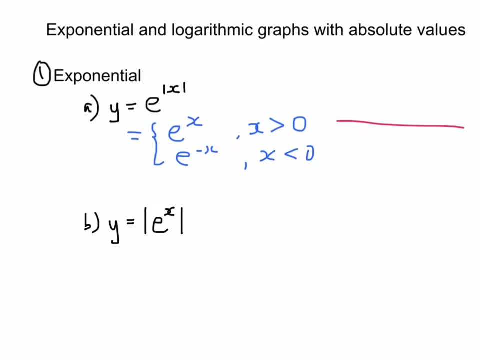 I knew I should, OK. So we've got the x and y axes as usual. And if I colour code these, if I make the bit on the right, the positive case, I forgot to make the little line there for the equals scenario. 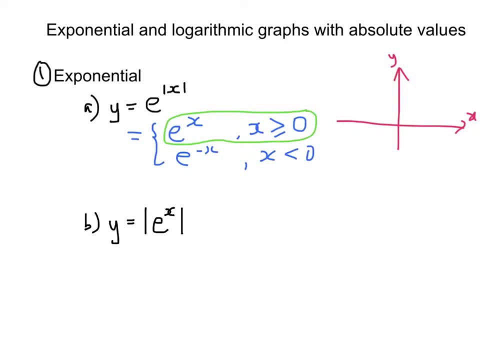 then it's going to be in a shape that's exponential, like so, except we only use this part of the graph, There we go, And it will have a y-intercept only, and it will be 0, 1.. Now, if you like, you can put this in. 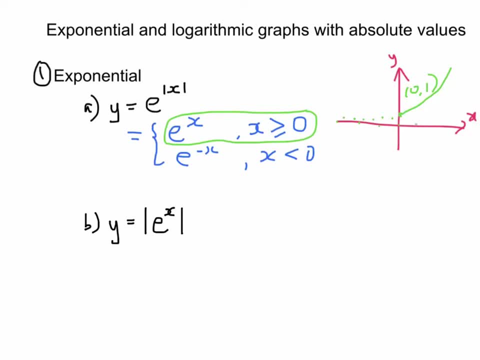 as a bit of more accurate detail, perhaps to explain what's going on. And so, if you do that, then you need to write in the y-asymptote, the horizontal asymptote, If we then colour code the left-hand side with, let's say, the purpley colour, 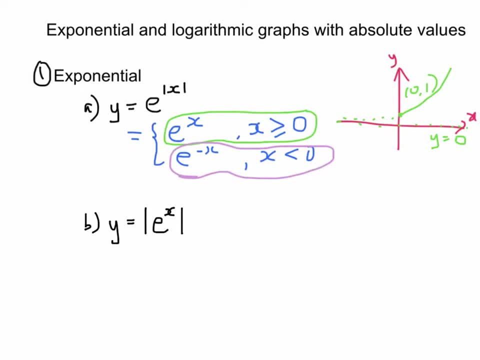 then this part of the graph will look like a reflected e to the x curve, reflected about the y-axis. So if that's the mirror, you get this shape over here, But you only pick the left-hand side values of the x-axis. 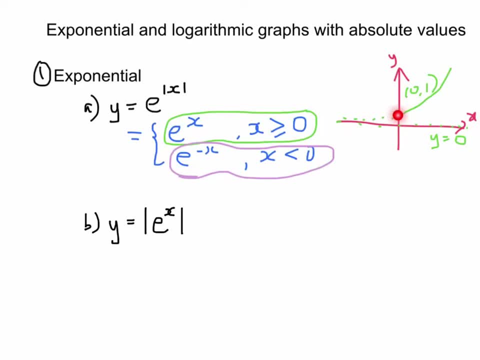 so we only have to draw in that part there. So you have this part here, And if you want it to be complete, then the rest of it would have been that dotted version. Now the second scenario: y is the absolute value of e to the x. 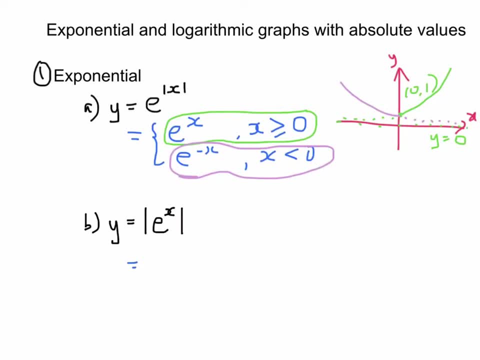 is actually a lot easier than you expect, because e to the x is positive for all x values. So this graph is actually the same as this graph here. So if I was to draw the basic graph on the right here- y and x- then your basic e to the x graph. 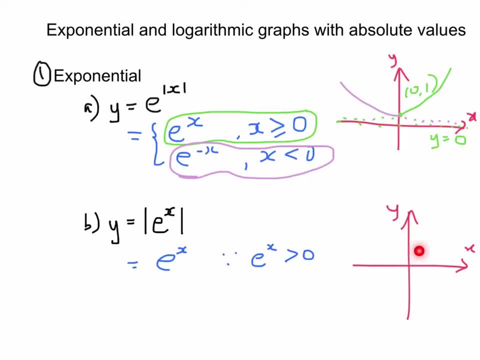 is shaped like this, And because it's always positive in the first place, then your final e to the x graph with the absolute value is actually the same. So I wrote that all funny, but I hope you get the idea. So now let's look at the logarithmic graphs. 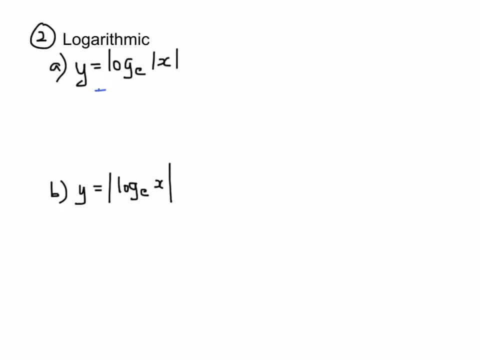 with absolute values. Again, we can write that in two parts. We can have the first part, which is where x is positive, So you keep everything the same for the case that x is greater than or equal to 0. Actually, you're not allowed to have that. 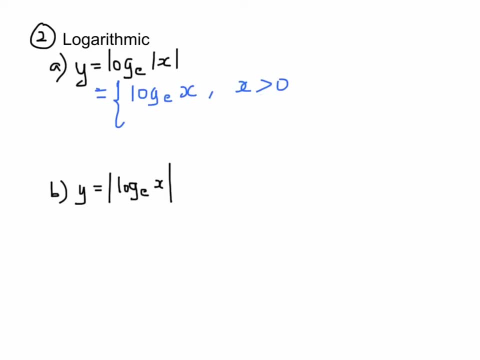 so I should just change that to x is greater than 0.. And the second scenario is where it's negative. So we would take the internal part of that bracket and multiply it by negative 1.. Now, if we draw this on a graph, 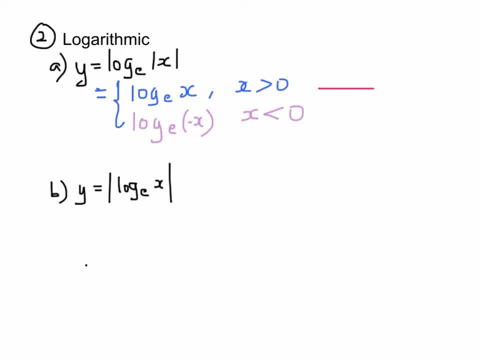 then what you have is the basic usual y and x axis and our basic graph of log e to the x itself has a vertical asymptote of x equals 0, and it has a shape like a banana. going that way And we'll have an x-intercept of 1, 0.. 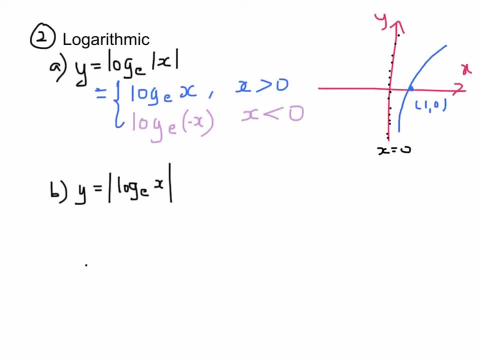 Now the reflected version would be looking at this, reflected horizontally, so that means it's reflected with this as the mirror line. so it's going to look like this. So if we draw that in, you'll have this shape here and you have the x-intercept at negative 1, 0.. 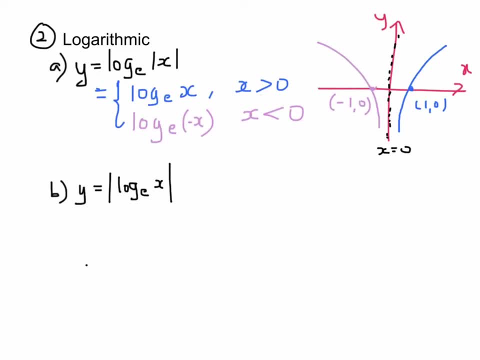 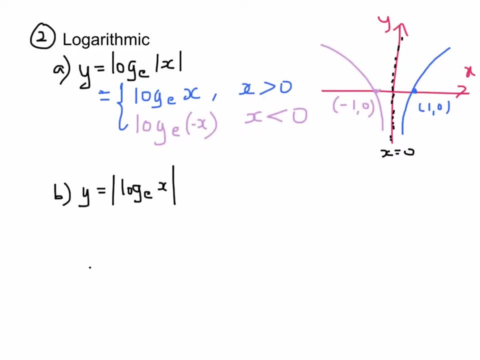 Now here's a second scenario where you have the absolute value of all of oops. this is the log e. there You're taking the absolute value of the whole thing. Now, the easiest way of doing this is to actually have the original sketch. 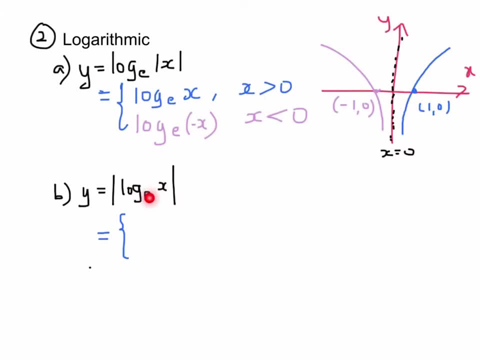 of what's in the actual bracket in the first place. So if I draw that over here, then the basic graph, it's colour coded with orange, of log e of x, is the banana shape going like this through here with a vertical asymptote of x equals 0,. 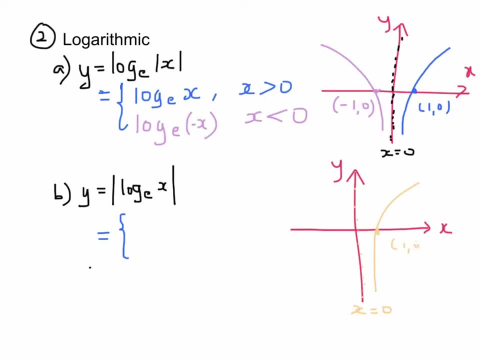 and it looks something like this: 1, 0 here. Now, knowing what we know about the absolute value, it means that you keep whatever is positive positive and you invert whatever is negative so that it's the negative 1 times that finite value. 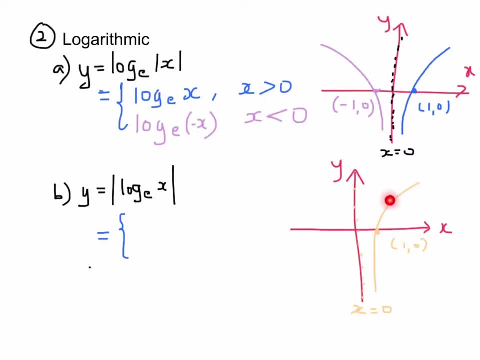 So on this part here it's positive in the first place. so we keep it as it is, and so we would write for this part: log to the base e of x if x is greater than 1, and we would draw that in blue over here like that. 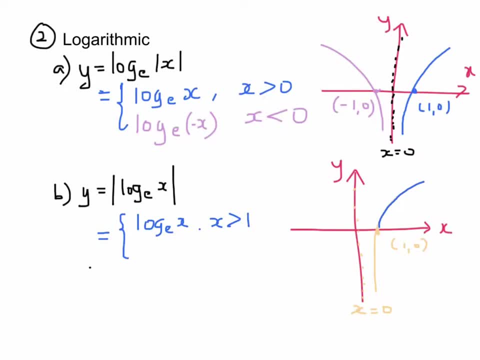 For the other part, it's where the graph is negative, which is between 0 and 1 in the x values. So we write that as negative log e of x where 0 is less than x is less than 1.. And it's not defined anywhere else. 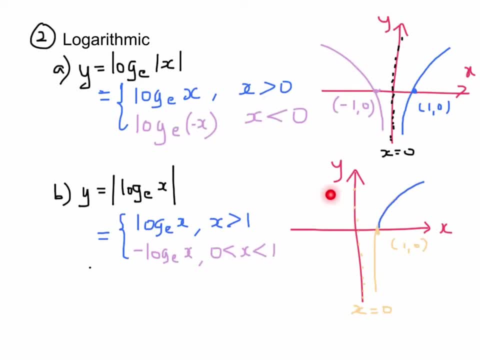 There's no possible values of this graph, for x is less than 0.. So to draw the final bit in, you'd take the reflection of this part and put it up here, So that will look like this: roughly, It'll still have the same x-intercept. 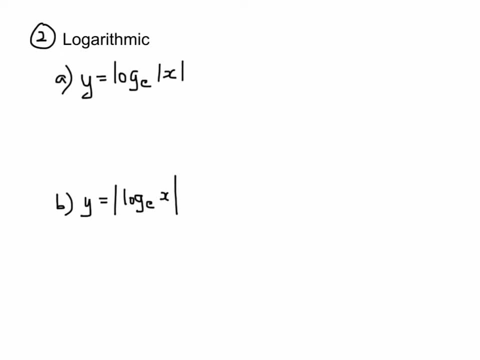 Now there is an alternative way of finding the rule and the inversion and all that sort of stuff for the second case. So let's say you blindly applied the rule where you could split that into two parts. You've got the positive case where log to the base e of x was positive. 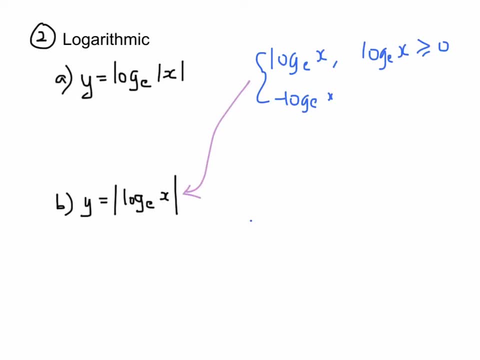 and the negative case where the log to the base e of x is negative. If we were to rewrite this part of the equation over here, that would be: log to the base e of x is greater than or equal to 0. And so you can make everything to the power of e. 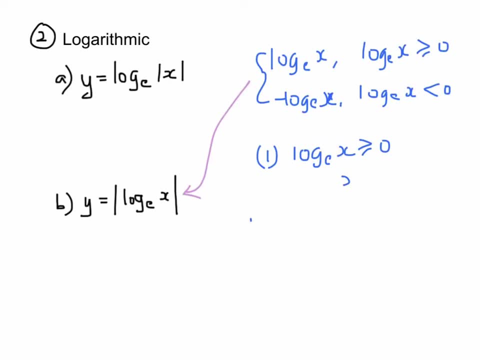 on both sides, which means you get rid of the log on this side to get: x is greater than or equal to e to the 0. And in case you forgot anything, to the power of 0 equals 1.. So this is a case where x is greater than or equal to 1.. 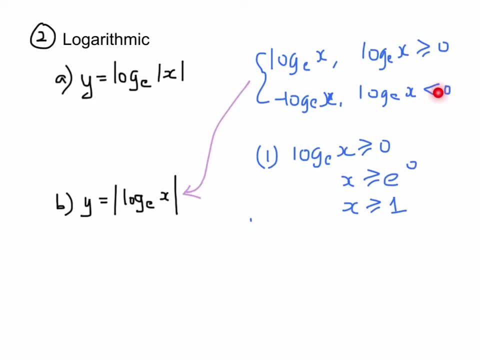 The second scenario here you can rewrite as log to the base: e of x is less than 0. And again the same algebraic tricks apply. So you'd still get: x is less than e to the power of 0, and so therefore x is less than 1.. 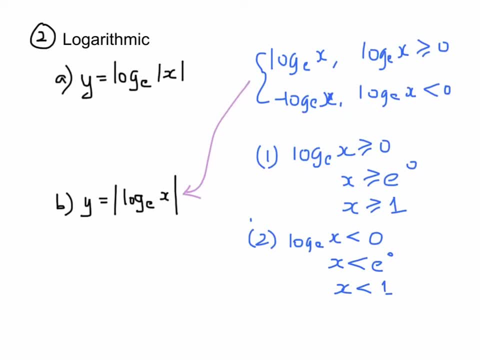 But you would have to recognise that we have to assume that this number here is greater than 0 for this to work. So therefore you have to actually know the second part here, that x is greater than 0, which is additional to what's actually in the equation. 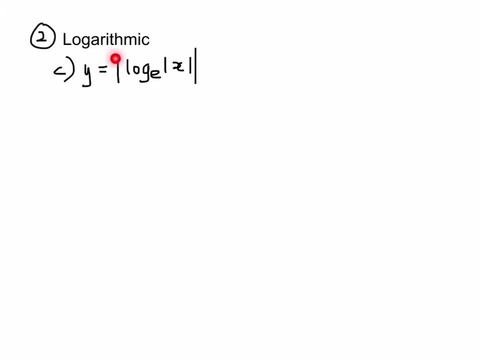 So here's one where you have an absolute value and another absolute value within that, And so what I do is actually split it into just drawing that first and then finding the absolute value later. So here's the sketch: Y-axis and x-axis. 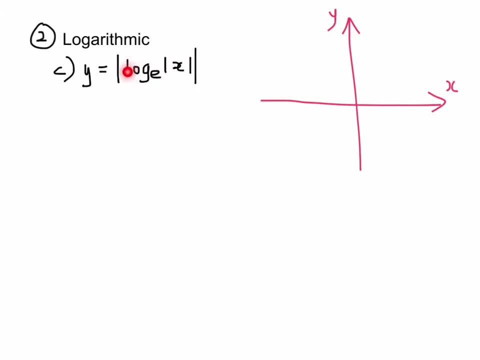 Now, this basic graph in here is actually the log graph on the right and the log graph reversed on the left, with intercepts of 1, 0, negative 1, 0 and an asymptote in the middle of x equaling 0.. 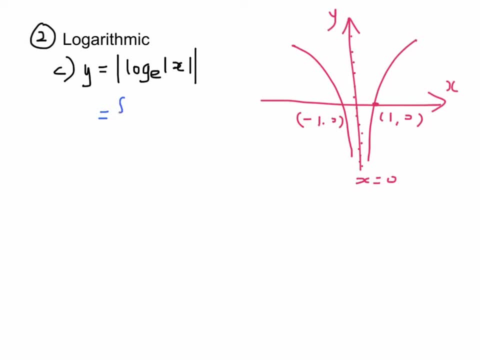 So we can split that up into the sections. In this case there are at least three sections: There's this section here, there's this section here, and the third section would be in between here and here. But because that's an asymptote, 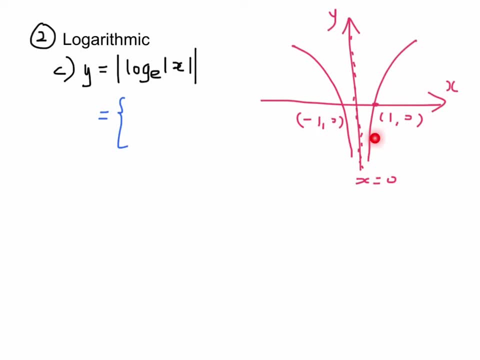 I can split that into two separate bits. So the convention is to write the positives first and then work your way downwards in the x values. So the first one is log to the base e of the absolute value of x, where x is greater than 1.. 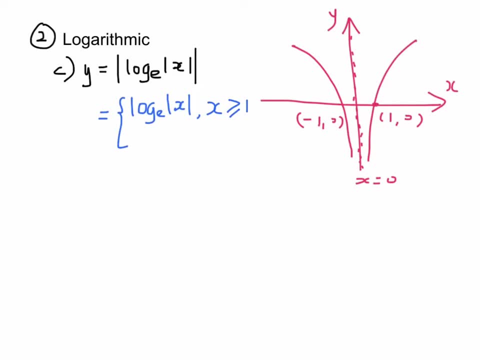 And I'll include the equal sign in there. So that will be this line over here. OK, Excuse this drawing. The next section is the negative section under here and that gets reversed up to there or reflected up to there. So I'll draw that in purple. 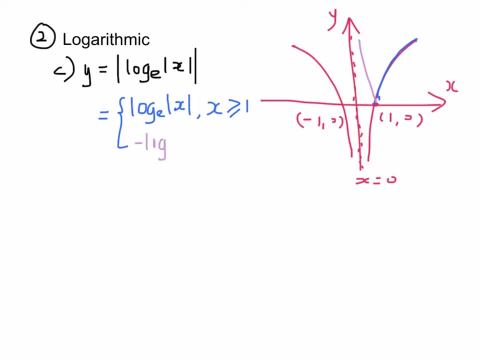 And if I write that in as the rule, we have negative log to the base e of x, where x lies between 0 and 1.. The next section is another purple section where you're looking at this negative region in here And so that gets reflected up here as well. 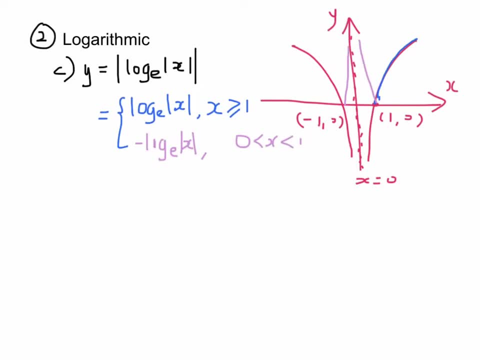 So we draw that in And there's still an asymptote of x equals 0. So the other scenario you could have is the same rule, but x is between 0 and negative 1. And we usually write the smaller number on the left. 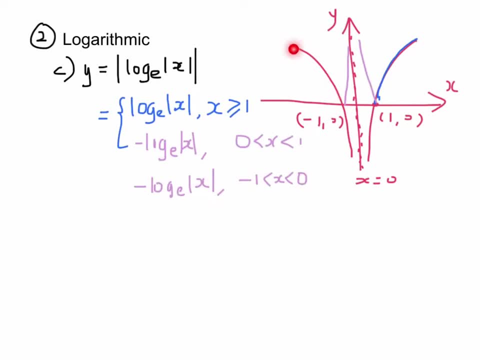 The last section is the positive over here And it's the case where x is less than negative 1.. So once again I'll draw it in in blue And the rule for that is: log to the base e of x where x is less than or equal to negative 1.. 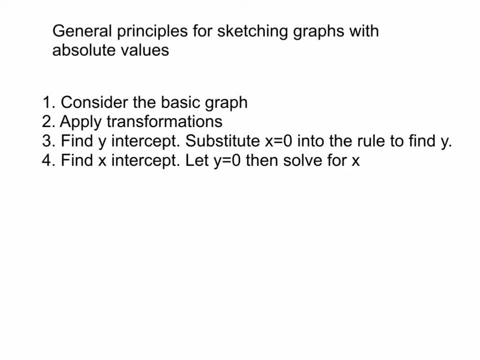 So here are some general principles. One: you have to consider the basic graph you've got. Two: you can apply transformations. Three: find the y-intercept by substituting x equals 0.. And four: find the x-intercept by letting y equal 0. 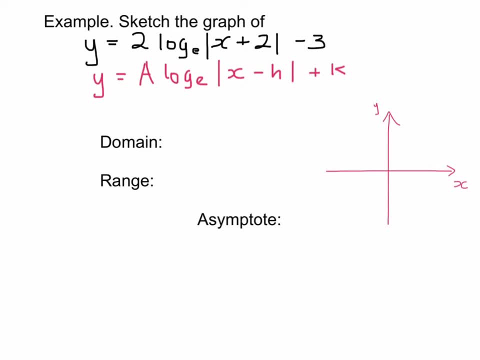 and then solving for x. So here's an example. Let's say we need to sketch the graph of 2 times log to the base e of the absolute value of x plus 2 and then take away 3 from that. So here's the general form of that graph. 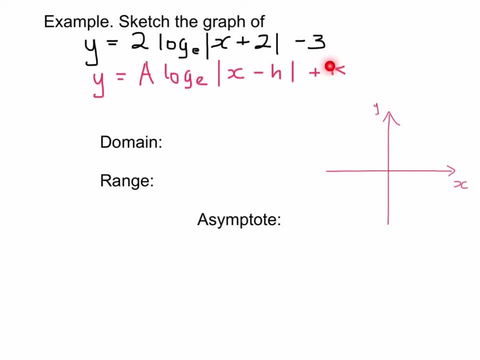 And hopefully you have remembered from before that this has a shape of what I look like as crutches or a funnel, perhaps centred at. x equals h As an asymptote. So if I look at this, what I have is a vertical dilation factor of 2.. 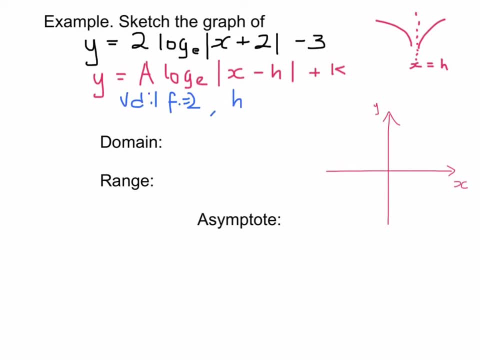 And we've got an h-value of negative 2, which means it moves 2 units to the left, And a k-value of negative 3, which means it's gone down 3. Which isn't really that much of a factor in log sketches. 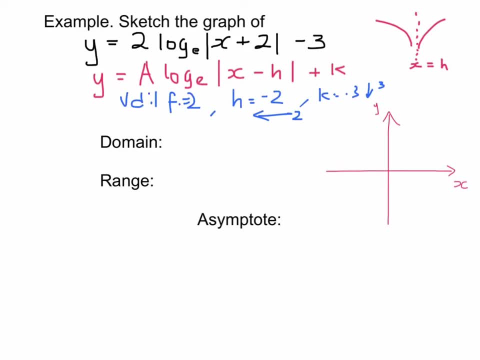 So what's our domain? Our domain is everything except for negative 2.. So we say x is not equal to negative 2.. Or you can say r with the backslash and then the curly brackets with a negative 2. there The range is r. 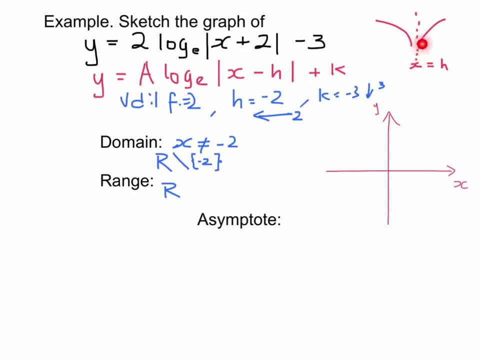 and hopefully you can see that, because it goes all the way down and up again. So our rough sketch. oh sorry, the asymptote is a vertical one. that's because it's logarithmic And the vertical asymptote is x equals negative 2.. 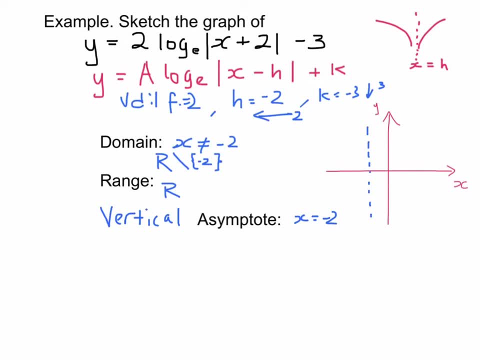 So we have a rough sketch of something like this so far. Actually, I forgot about the horizontal- oh sorry, the vertical- movement, So it's more likely to be shifted downwards by 3 units, so it might be perhaps something like this. So you have to be prepared for any eventuality. 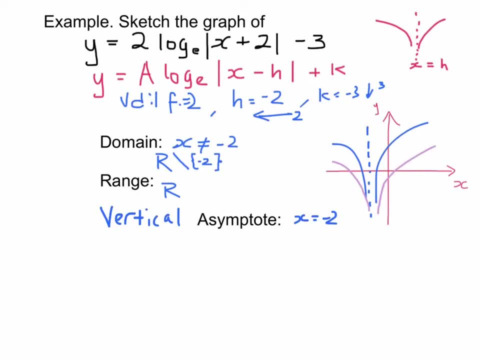 You're still going to get the same number of x-intercepts- 1 and 2, or 1 and 2, depending on the shape- And you're still going to get one y-intercept in either case. So let's see what we get. 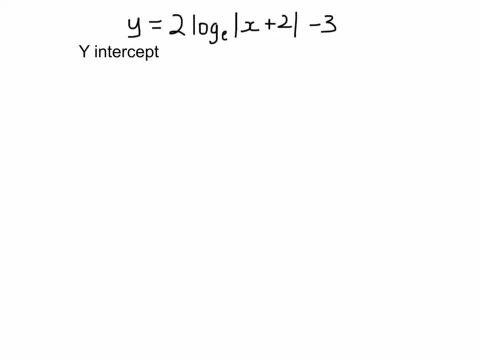 So let's find the y-intercept. To do this, we let x equal to negative 2.. To do this, we let x equal 0. And then work out what y is. So y equals 2. log to the base e of 0 plus 2 minus 3.. 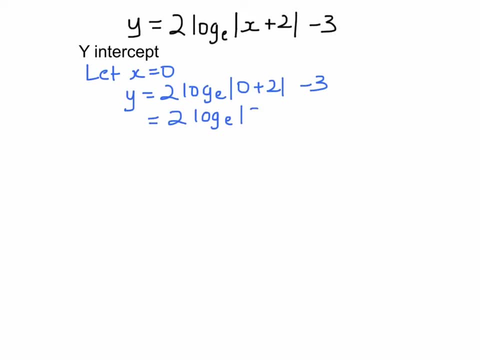 So that equals 2 times log to the base e of the absolute value of 2, take 3.. Now 2 is already positive, so you keep it as it is. So you have 2 log e to the log to the base e. sorry, 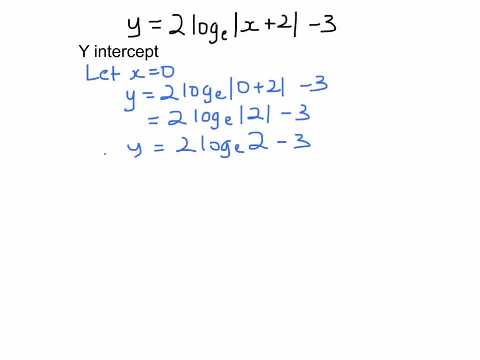 2, take away 3 as your y-intercept, So you can write that in exact form as 0, 2 log e, 2 take away 3.. Or, if you use a calculator, it's approximately equal to 0 negative 1 point 6, 1. 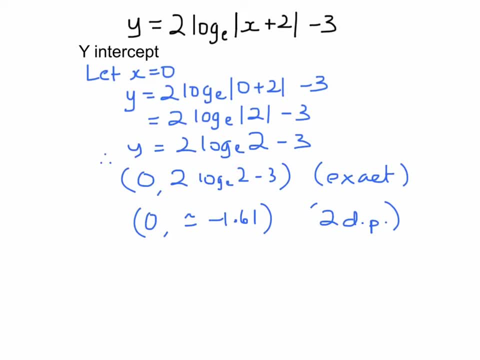 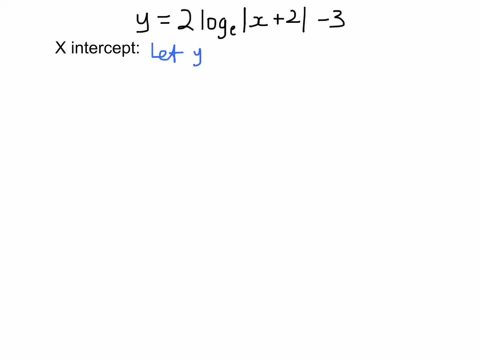 if you're writing it correct to 2 decimal places. Next we'll work out the x-intercepts. And to do that you let y equal 0. And then solve for x. So 0 equals 2. log to the base e of x plus 2. take away 3.. 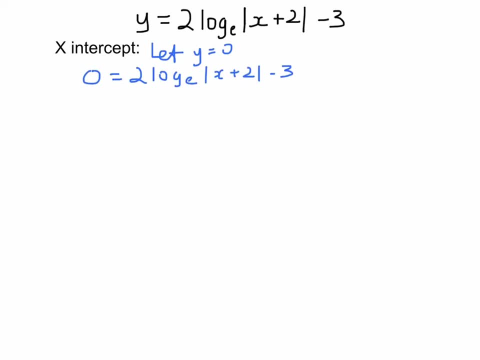 And our first step is to get rid of the take away 3 by adding 3 to both sides, So that gives you 3 equals 2. log to the base e of x plus 2.. We can then divide by 2, so you get 3 over 2. 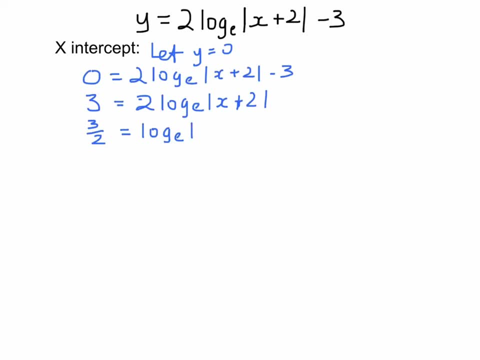 equals log to the base e of x plus 2 in absolute value terms. And then here we just use the same tricks as before: We have to raise everything to the power of e, So that becomes e to the power of 3 halves and leaves behind this absolute value thing. 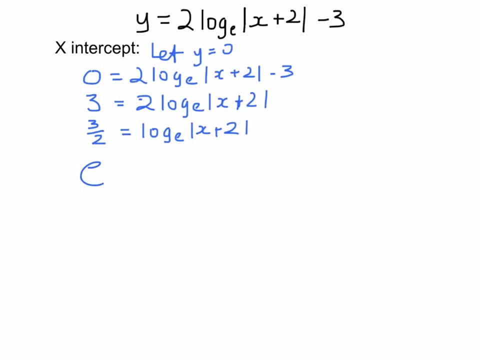 So what we have is: e to the power of 3 on 2 equals the absolute value of x plus 2.. So now we have two possible scenarios. Scenario 1 is where the absolute value of the contents of the absolute value are positive. 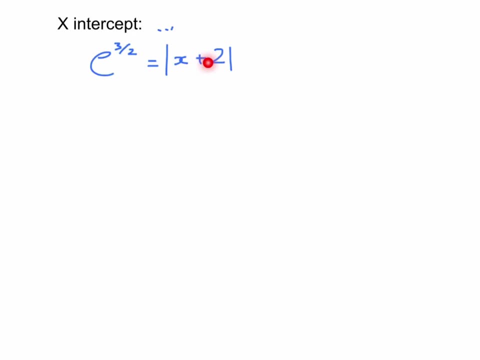 And scenario 2, where the contents are negative. So we'll split them in half, like so Here we'll have: if the contents of the absolute value are positive, then it equals to e, to the power of 3 over 2, equals x plus 2.. 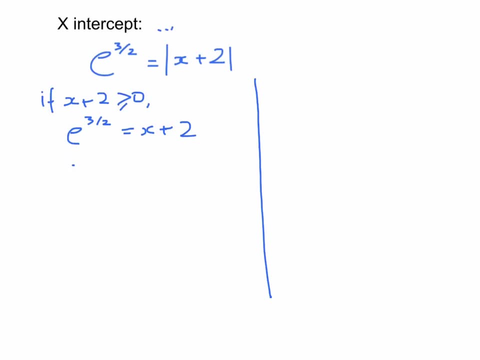 And if we solve that for x, we get x is equal to e, to the power of 3 on 2, take away 2.. That's the exact version, The approximate version you'd get from your calculator, which gives you 2.48.. 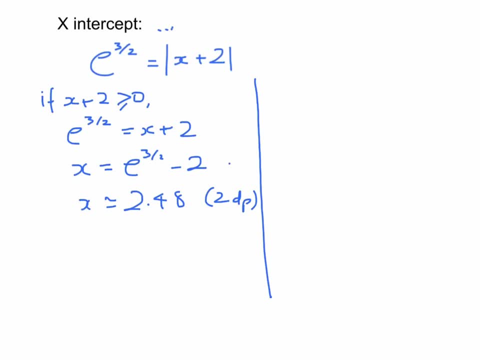 That's correct at two decimal places. Now this actually corresponds to x being greater than or equal to negative 2.. So that actually matches, because 2.48 is bigger than negative 2.. Now the second scenario is where the contents of the absolute value 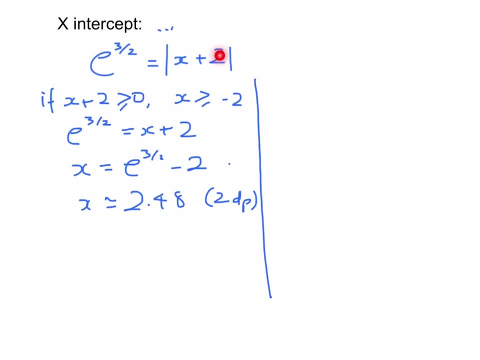 are negative. So we have: if x plus 2 is less than 0, then e to the power of 3 on 2 is equal to the negative 1 times x plus 2.. And that gives you negative x minus 2.. Which then you can solve for x. 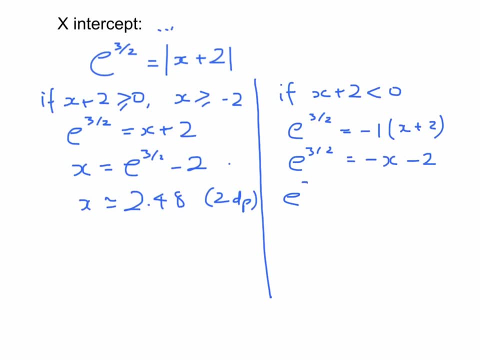 by adding 2 to both sides. So you get e to the power of 3 on 2 plus 2 equals negative x. And then, last but not least, you divide by 2.. You could have divided by negative 1 before, but I chose to do the expansion. for some reason. 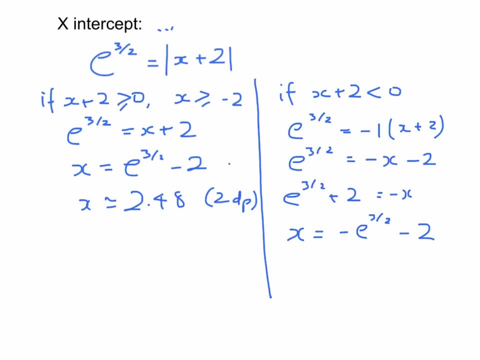 Equally fine for both reasons. So that approximately equals negative 6.48 to two decimal places. So to clarify, if I was to look back here this would give me: x is less than negative 2.. x is less than negative 2.. 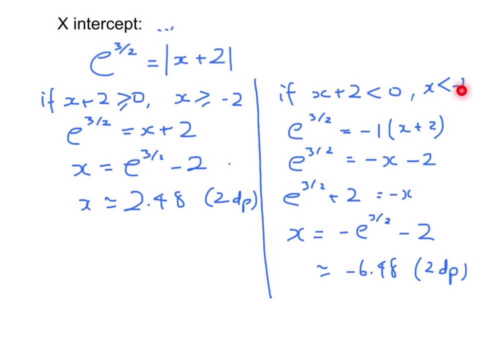 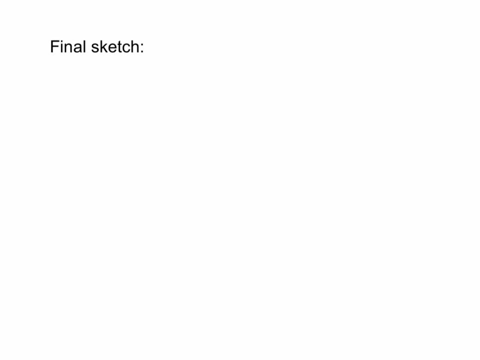 And that makes sense. It matches up because negative 6.48 is indeed smaller than negative 2.. So here's how I do my final sketch. I know that I have a shape, something like this, And the asymptote is: x is negative 2.. 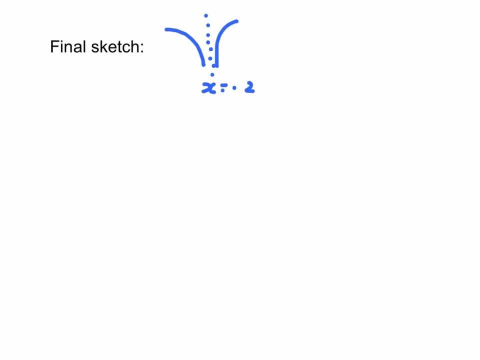 What else do we know? And we know from previous work that the y-intercept is 0 comma, negative 1.61 approximately, And the 2 x-intercepts are 2.480 and negative 6.480.. So this helps me to draw my axes. 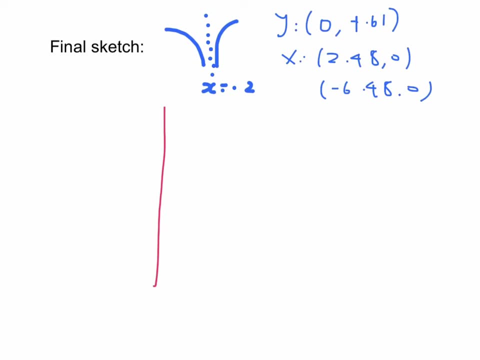 and therefore sketch my graph in the right spot. So here's the approximate version. My asymptote at x equals negative. 2 is over here, And if I put my y-intercept in it's going to be negative down here somewhere. And if I put my 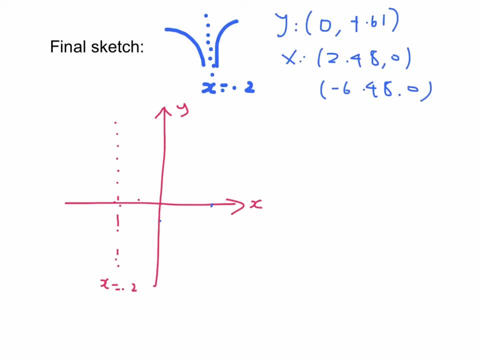 x-intercept of 2.48. it's going to be slightly over here, like that, And negative 6 is way over off the scale somewhere, So something like this is good enough. It looks pretty bad actually, but I'm looking as a maths. 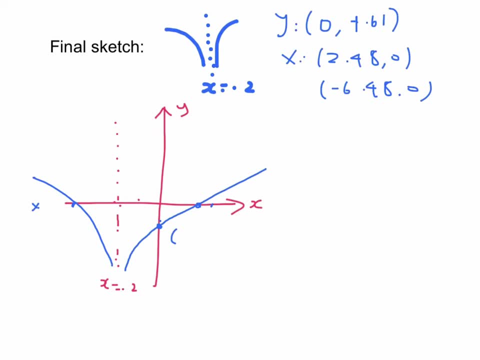 marker for whether you've put the labels in the right spot. So you go 0, negative 1.61, and this one will be 2.48 comma 0.. And this one is negative: 6.48 comma 0.. Now if, for some reason, 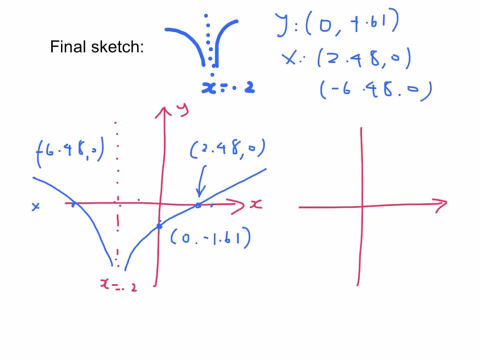 you are not asked to round anything to any decimal places, then that means you have to put everything to exact form. Now, that's a terrible line, but you get the idea that that's an asymptote And I would pay that because I've labelled it. 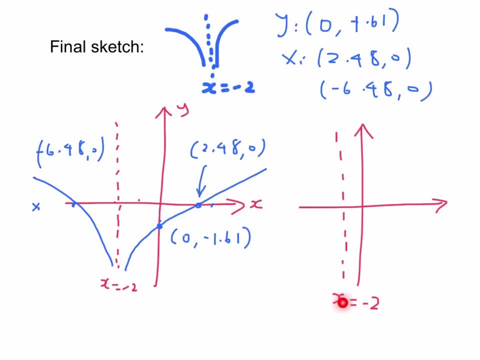 So that's the marking there And I would be looking as a marker for whether you've marked in your intercepts as coordinates. Now, if we're going to put in exact form, this one would have coordinates of 0 and what was it? 2ln2.